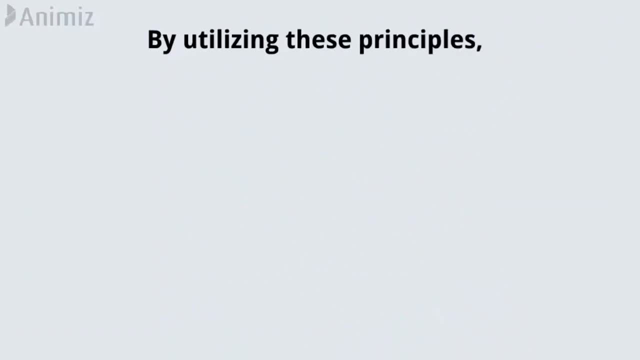 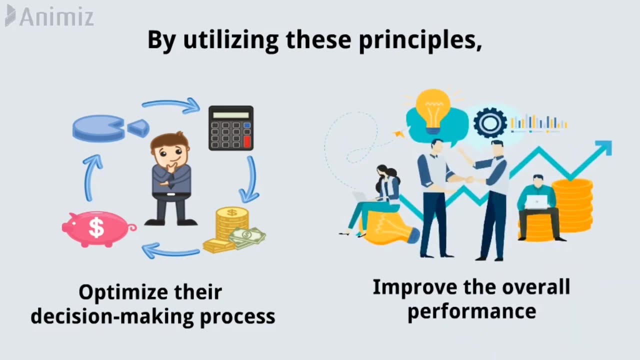 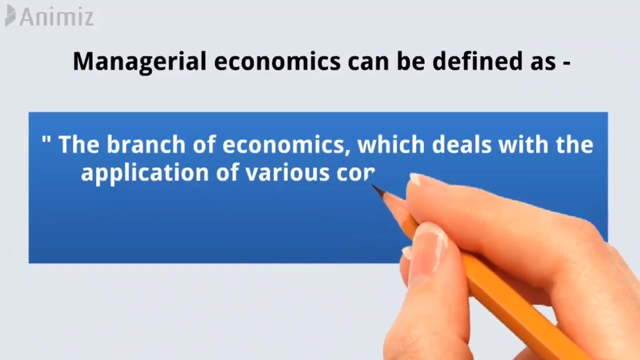 business problems. By utilizing these principles, managers can optimize their decision-making processes and improve the overall performance of their organizations. So managerial economics can be defined as the branch of economics which deals with the application of various concepts, theories, methodologies of economics to solve practical 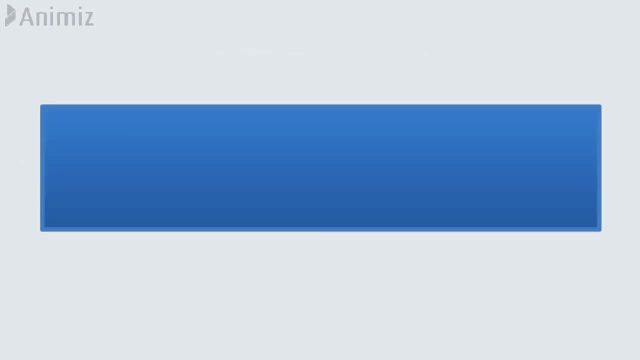 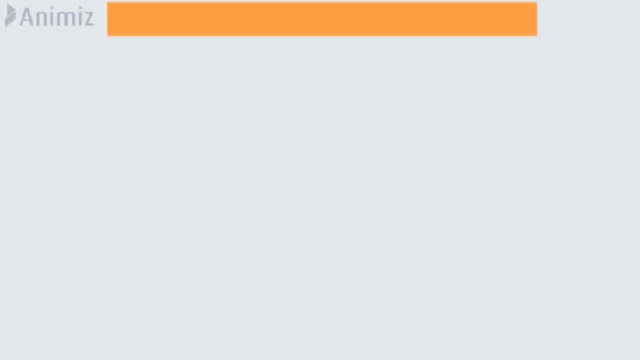 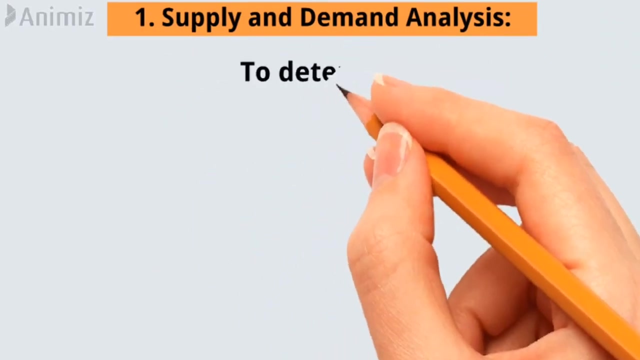 problems in business management. Let's dive into some key concepts of managerial economics that empower managers to make informed decisions. Number 1. Supply and Demand Analysis: Understanding the Forces of Supply and Demand Analysis. Understanding the Forces of Supply and Demand is necessary for businesses to determine optimal 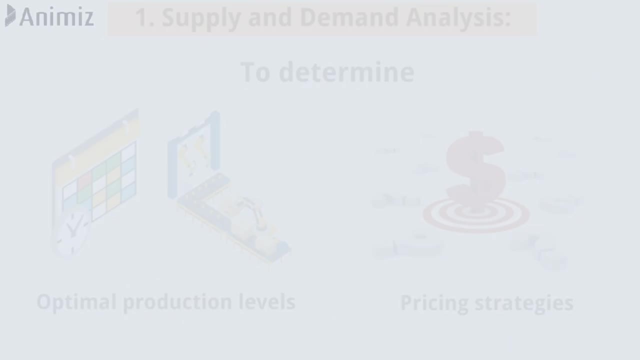 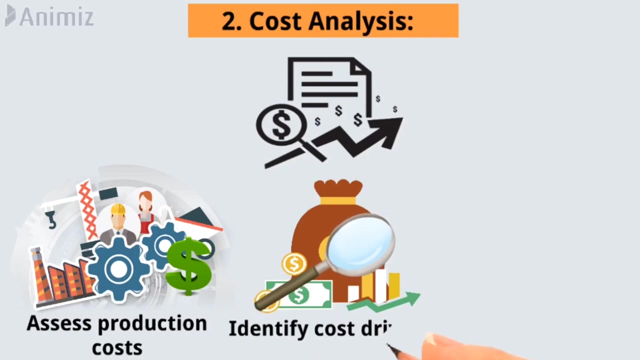 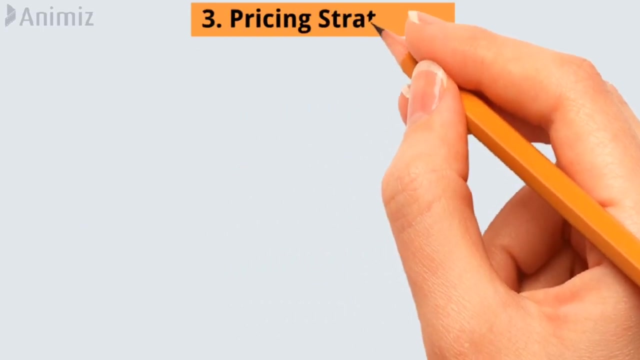 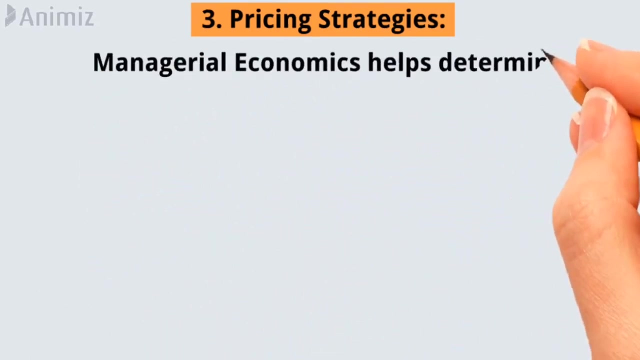 production levels and pricing strategies. Number 2. Cost Analysis. Cost analysis helps managers assess production costs, identify cost drivers and make informed decisions about resource allocation. Number 3. Pricing Strategies. Setting the right price is a critical decision for businesses. Managerial economics helps determine optimal pricing strategies. 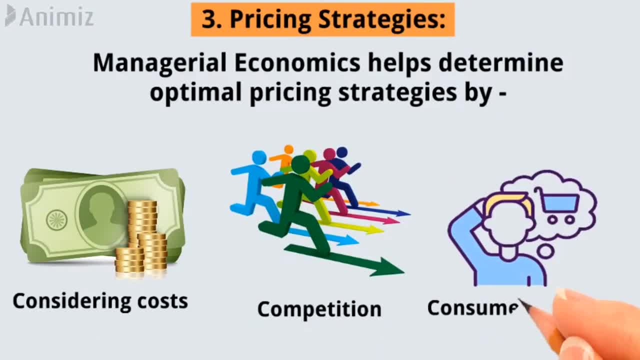 It is important to understand the right pricing strategy by considering costs, competition and consumer behavior. The pricing strategy is a critical step in understanding the election fears and the market overall market. The price-to-market pricing strategy is one of the few tools that help to understand the 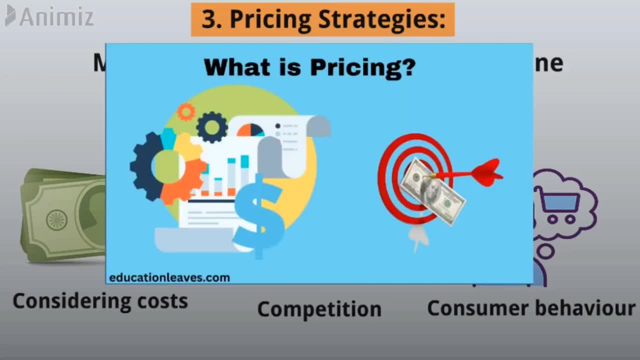 cost, efficiency and behaviour of the markets. I have discussed in detail the pricing strategy in a separate video. Check that video link in the description. you'll find the pricing strategies in the description. We can see the pricing strategies listed throughout the video. 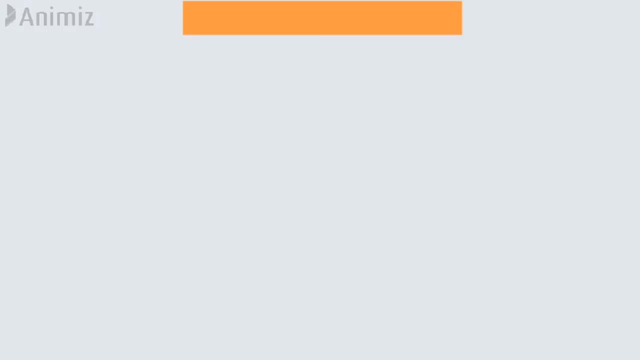 In addition, we have a separate video on the pricing strategy. If you want more information about pricing strategies, check out our video on pricing strategies in the description Number 4. Marketing Principles: Understanding different market structures, such as perfect competition, monopolistic competition. 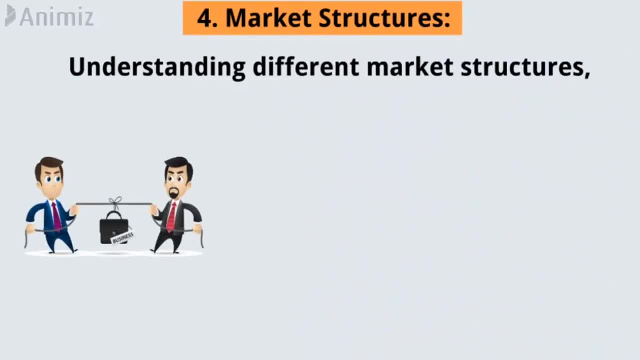 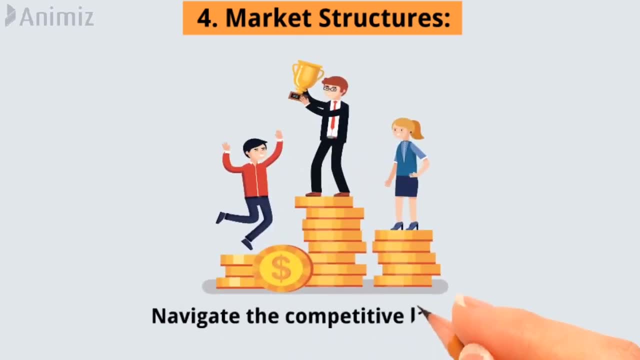 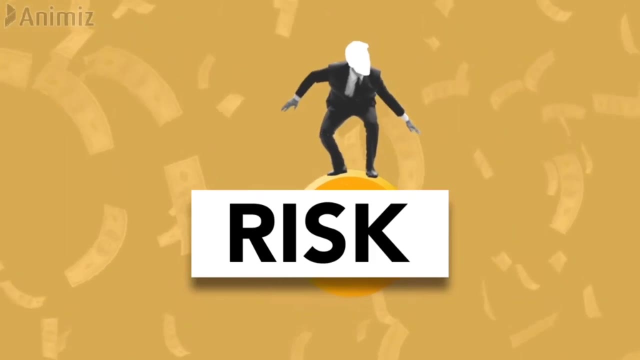 oligopoly, et cetera, enables managers to navigate the competitive landscape effectively. different market structures, such as perfect competition, monopolistic competition, oligopoly, etc. enables managers to navigate the competitive landscape effectively. 5. Risk Analysis: Business decisions involve inherent risks and uncertainties. 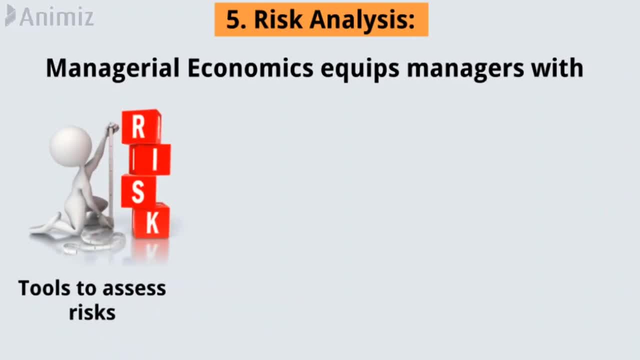 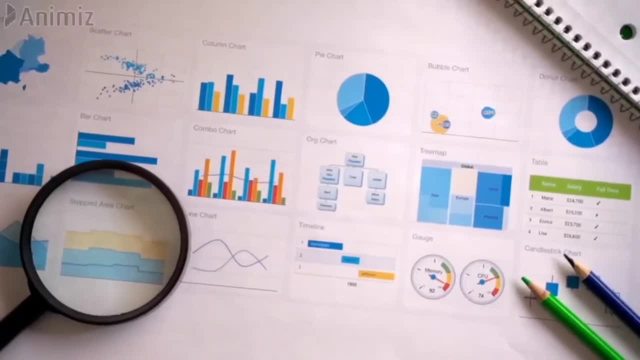 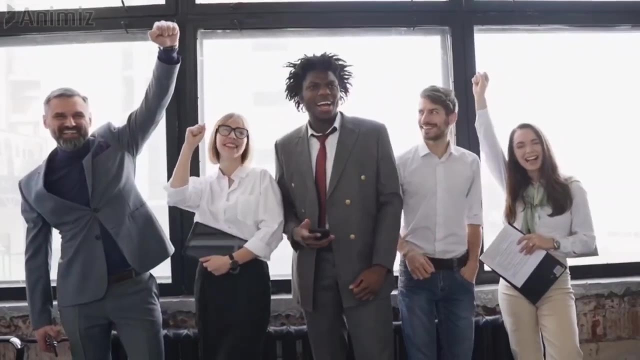 Managerial economics equips managers with tools to assess risks, make informed judgments and develop contingency plans. By integrating these concepts into their decision-making process, managers can gain a competitive edge and drive their organizations towards success. Also, some economic principles that managers should keep in mind. 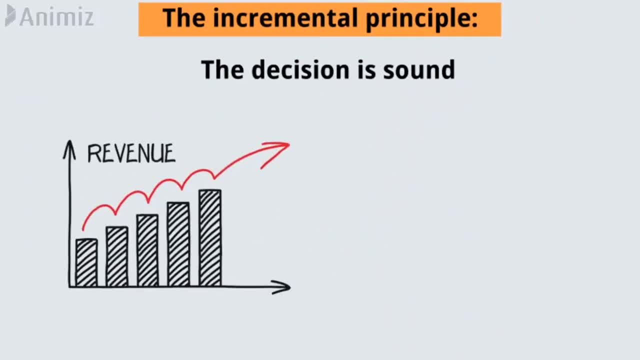 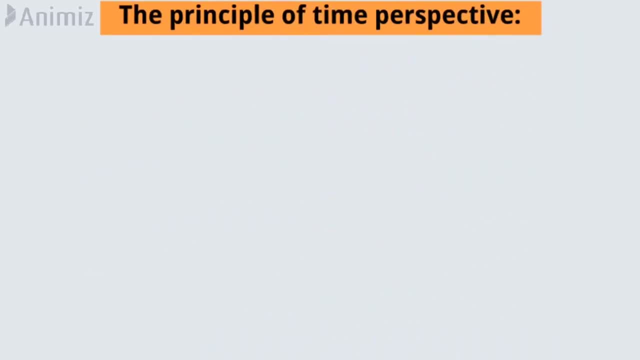 The incremental principle: The decision is sound if it increases revenue more than cost or if it reduces cost more than revenue. The principle of time perspective: A decision should take into account both the short-run and long-run effects on revenue and cost, giving appropriate weight to the most relevant time period in each individual decision.